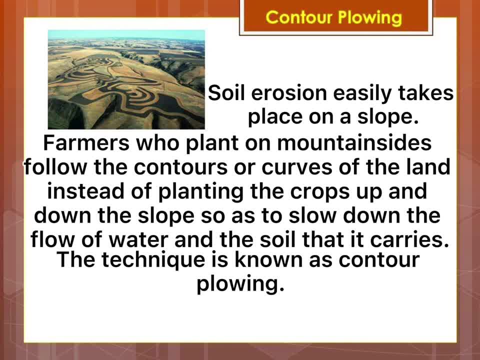 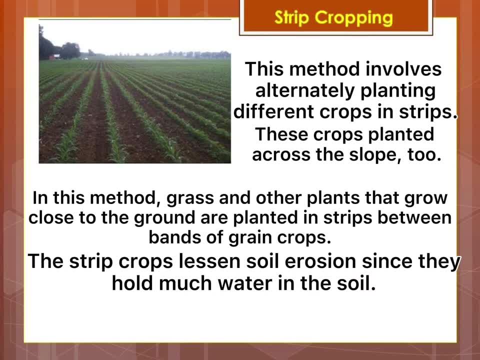 Water. Water is used to slow down the flow of water and the soil that it carries. The technique is known as contour plowing, Strip cropping. This method involves alternately planting different crops in strips. These crops planted across the slope too. In this method, grass and other plants that grow close to the ground. 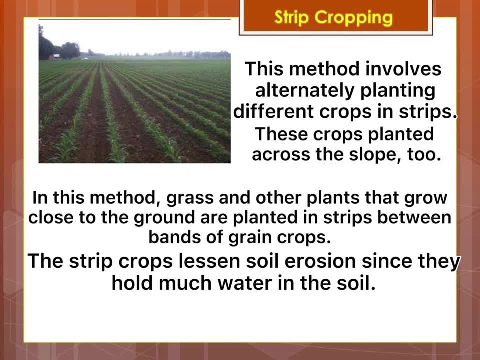 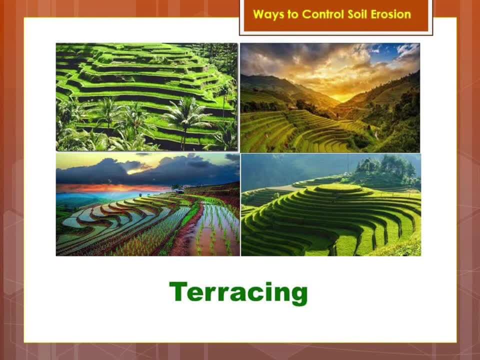 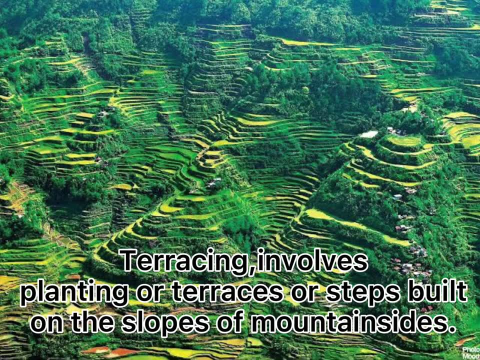 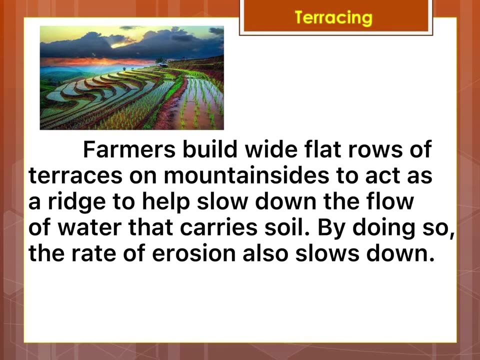 are planted in strips between bands of grain crops. The strip crops lessen soil erosion since they hold much water in the soil Water. next we have terracing. terracing involves planting or terraces or steps built in the slopes of mountainsides. farmers build wide, flat rows off terraces on mountainsides to act as a ridge to. 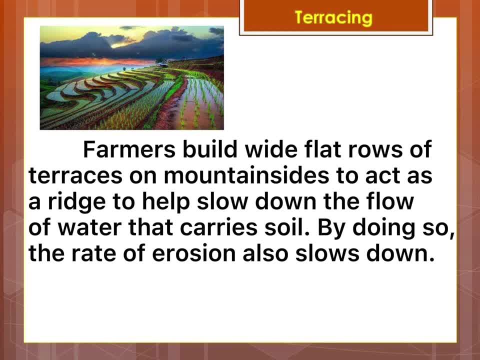 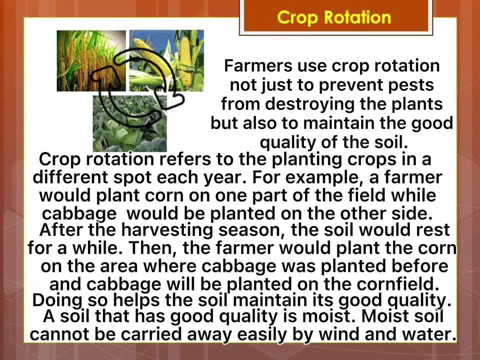 help slow down the flow of water that carries soil. by doing so, the rate of erosion also slows down crop rotation. farmers use crop rotation not just to prevent pests from destroying the plants, but also to maintain the good quality of the soil. crop rotation refers to the planting crops in 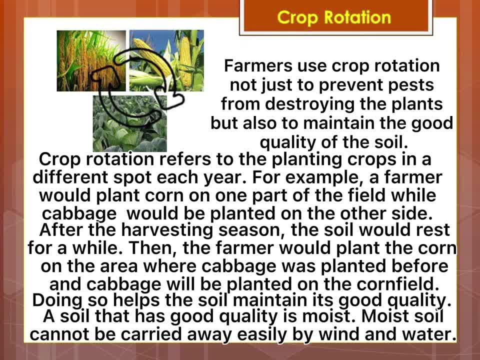 a different spot each year. for example, a farmer would plant corn on one part of the field, while cabbage would be planted on the other side. after the harvesting season, the soil would rest for a while. then the farmer would plant the corn on the area where cabbage was planted before and 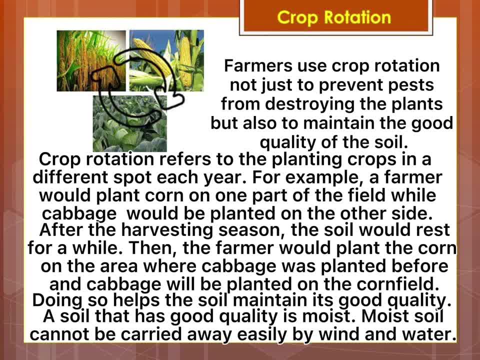 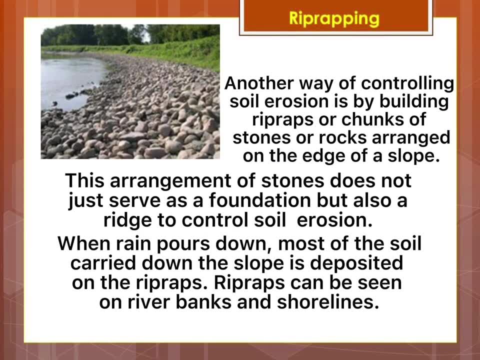 cabbage will be planted on the cornfield. doing so helps the soil maintain its good quality. a soil that has good quality is moist. moist soil cannot be carried away easily by wind and water reprapping. another way of controlling soil erosion is by building repraps or chunks of stones or rocks. 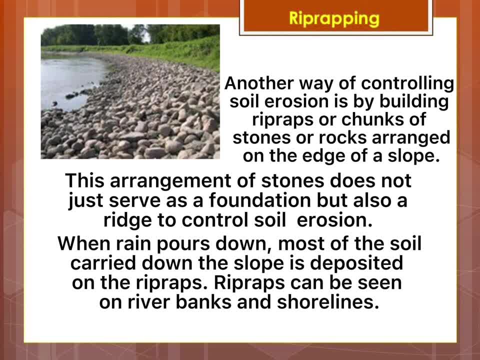 arranged in the edge of a slope. this arrangement of stones does not just serve as a foundation, but also a ridge to control soil erosion. when rain pours down, most of the soil carried down the slope is deposited on the reprapping. repraps can be seen on riverbanks and shorelines how forests help in controlling soil erosion. 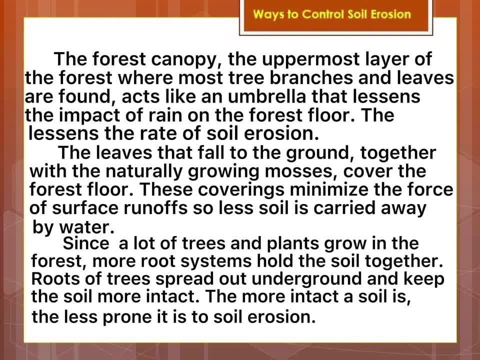 the forest canopy, the uppermost layer of the forest, where most tree branches and leaves are found, acts like an umbrella that lessens the impact of rain on the forest floor. the lessens the rate of soil erosion. the leaves that fall to the ground, together with the naturally growing.